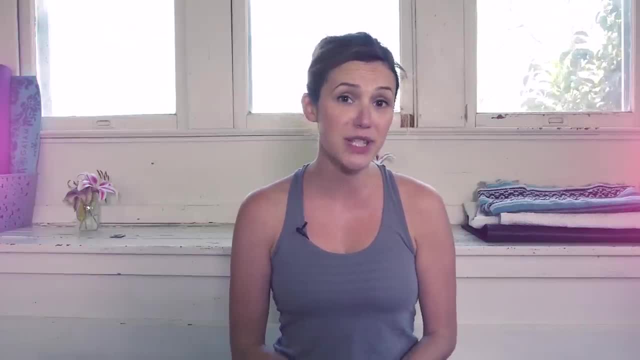 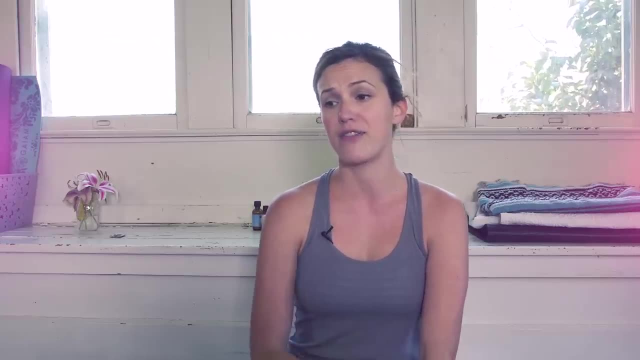 Hey everyone, welcome to Yoga With Adriene. I am Adriene and today we have a sequence for the lower back. This is something that you requested and I think is awesome and really dear to me, because I very much believe in the healing power of yoga practice. keyword: 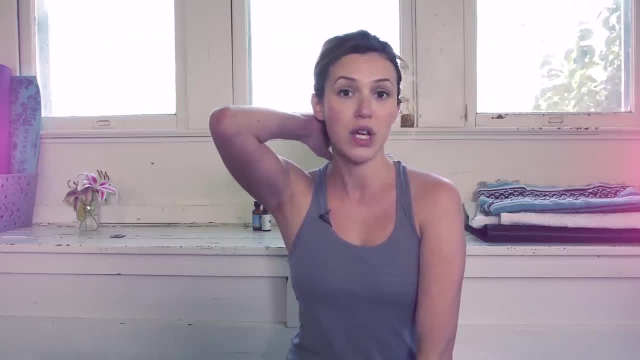 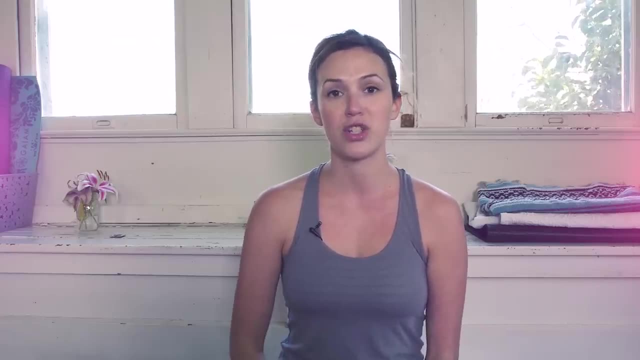 practice. So I encourage you, invite you, to try this video more than once. Embrace the repetition. You might favorite the video or click the add to tab below so you can find it more easily. But this is something that I think, if you practice regularly, will really. 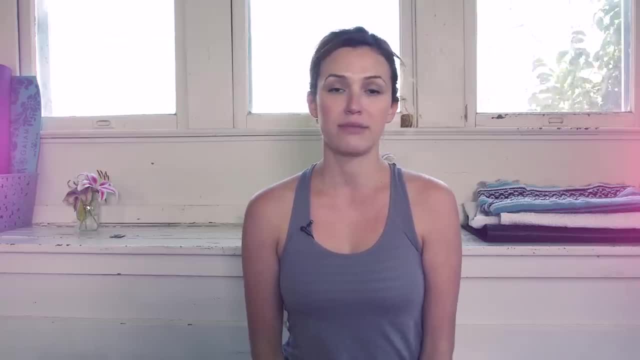 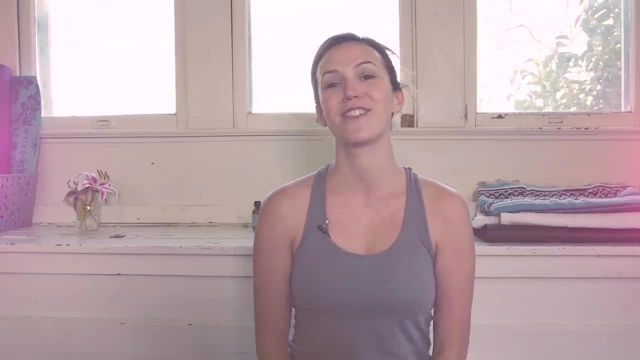 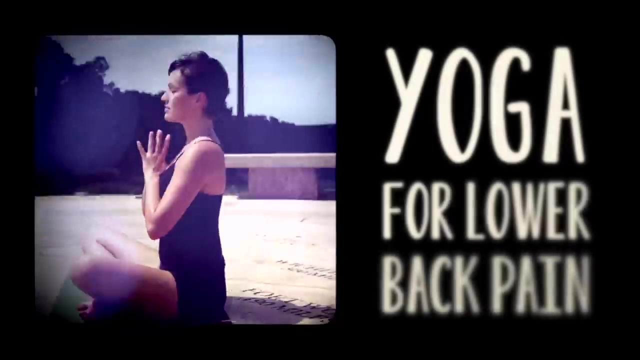 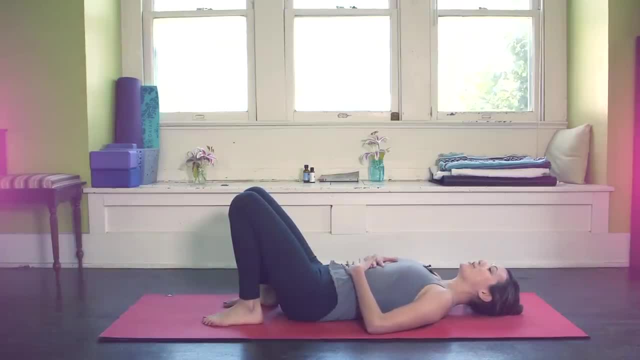 going to start flat on our backs today, using the support of the earth to tend to the lower back. I just love all poses on the back because it reminds me that we are supported. So if you want to go there with me, if you want to go, oh, nevermind, I can't sing that explicit. 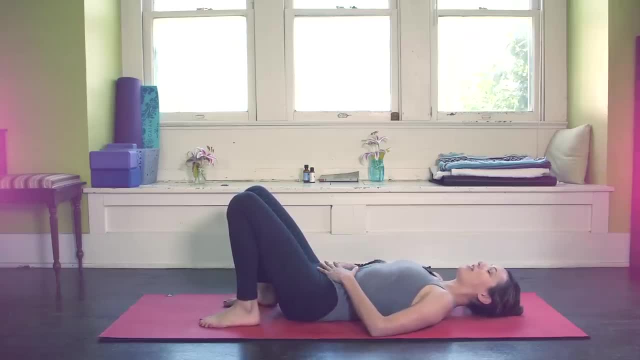 lyrics. If you want to go there with me, you can just kind of take a deep breath in and already just feel relief from the idea that we are supported by the mat, by the earth. By this moment I feel like a little bit of consciousness goes a long way. 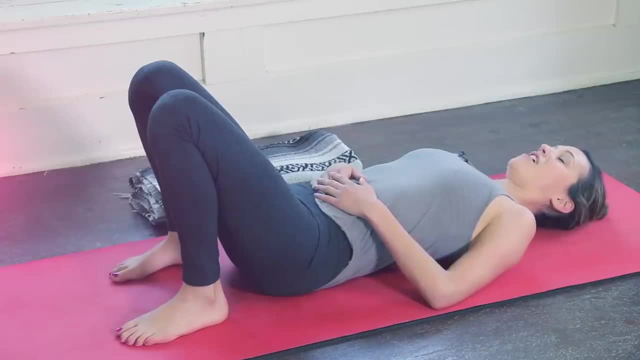 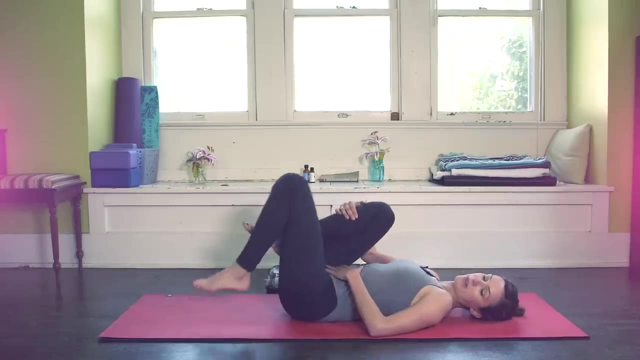 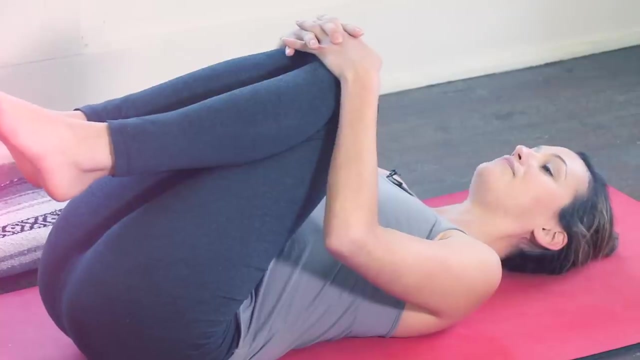 So take a deep breath in, long, exhale out And slowly we're going to wrap the arms around the shins, might interlace the fingertips here And nice and slow we'll let the knees come in towards the heart. So if the lower back is already starting to talk to you, you have a couple options. 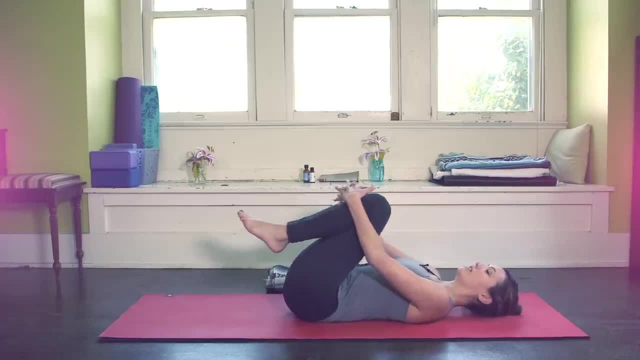 Those can come to the knees. this is great. or again, we can interlace. Now, rather than hardcore squeezing, just breathe here, relax the shoulders down, let the weight of the elbows drop, And we have two options. We're going to rock a little side to side, just kind of massaging the lower back, not. 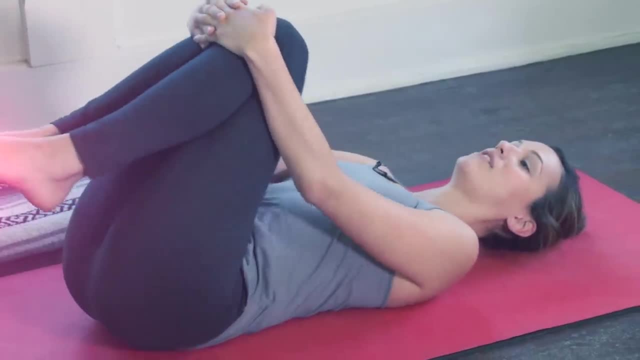 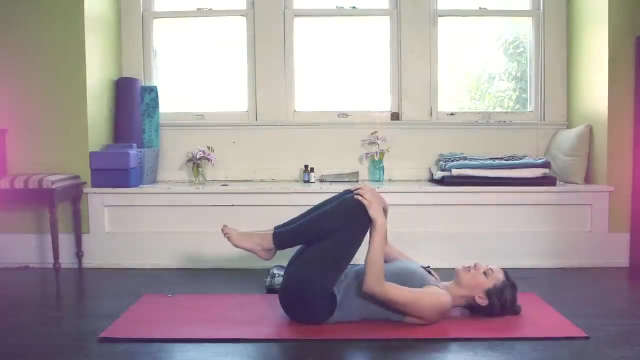 squeezing like I do normally in Hatha Yoga, but just kind of letting the space be. So I have an option here, or I have the option to draw circles with the palms. So just take a second here on your own, Because everyone's different. 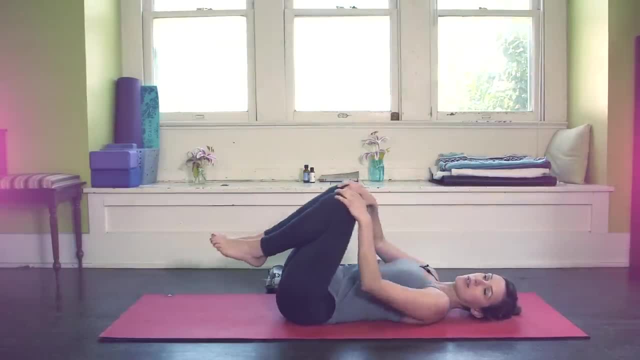 It's so hard to do yoga for this and yoga for that, because everyone's different, everyone's experiencing different sensations. So just try to honor that And I'll encourage you to listen to your body, be gentle and, of course, modify up, modify. 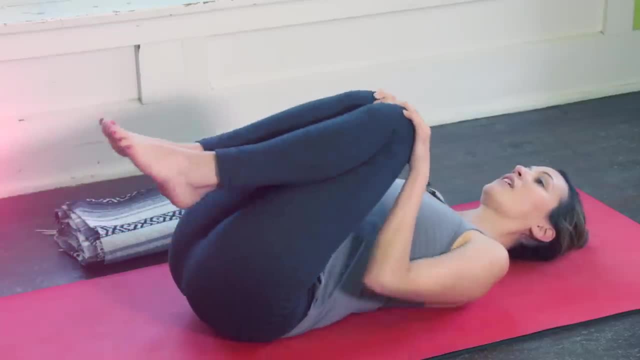 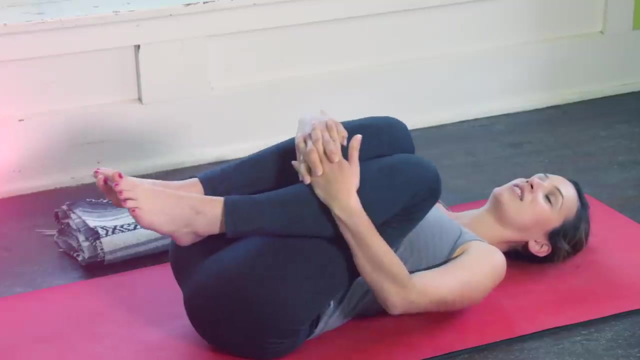 down as needed. So what we're doing is drawing circles with the palms on the knees one way and then the other, Or where fingertips interlace, Fingers interlace going left to right might even linger on one side, if that feels good. 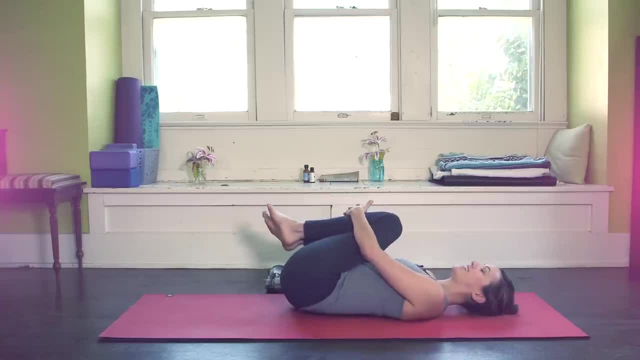 And then close your eyes, look away from the video and just take a second to feel both these things out. So check in with the lower back, Make sure you're breathing deep, Awesome. Then, when you feel satisfied, slowly We'll release the soles of the feet to the mat. 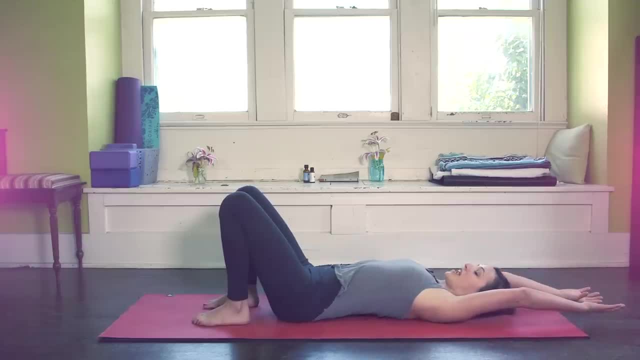 And we'll inhale, reach the fingertips all the way up and overhead. Nice and easy. We're going to just rock the pelvis here. So I'm going to rock the pelvis so that the lower back becomes kind of a rainbow over. 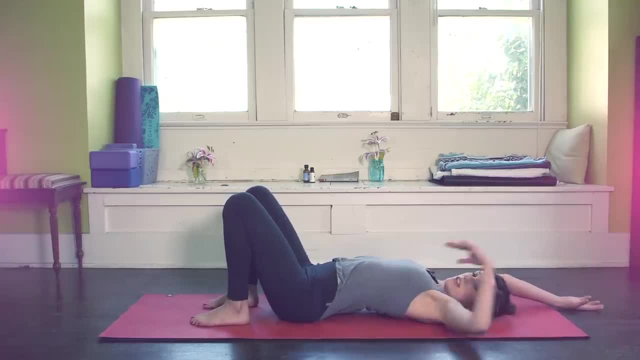 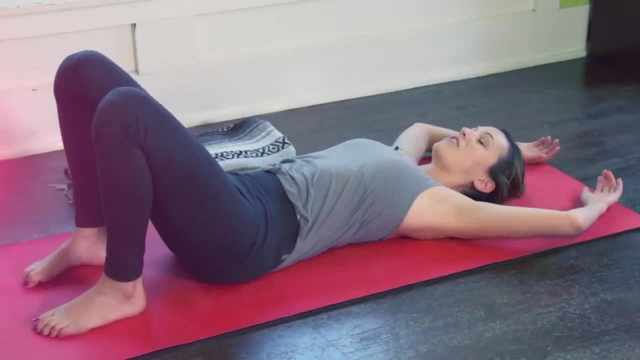 my mat, So if I wanted, I could slip my hand underneath there. And then I'm just going to rock the pelvis here. Get sassy. So nice and easy. We can bend the elbows as I tuck the pelvis. 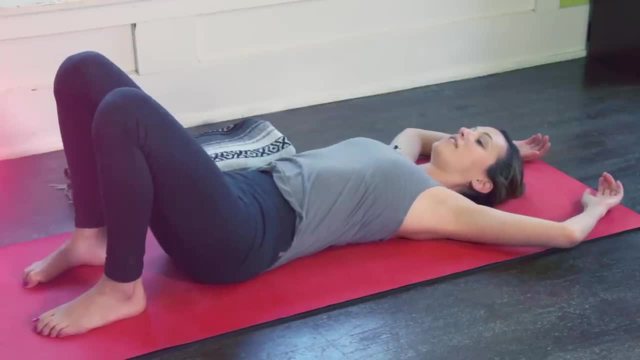 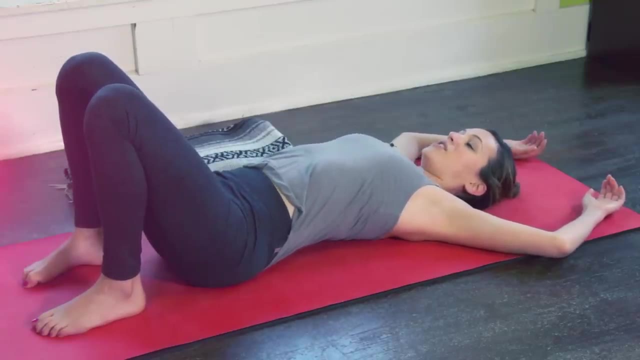 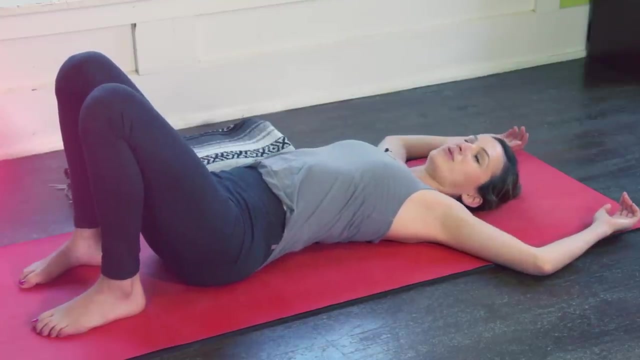 And then I'm just going to rock the pelvis here, Get sassy And then exhale tailbone down, navel stretches long, belly stretches long, And then we switch. Doesn't even matter what you're inhaling on and what you're exhaling on. 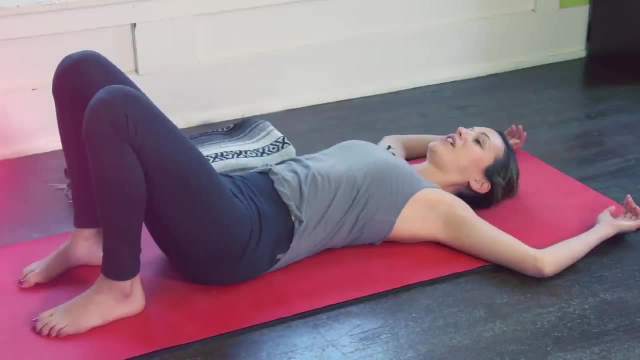 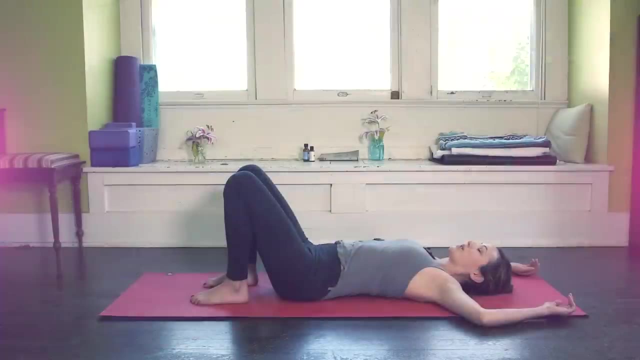 Just breathe deep And I'm sure this is going to look great on the video. but we're just kind of coming into almost a little sensual pelvic rock here. But it's awesome because we're massaging the top of the buttocks here and we're just loosening. 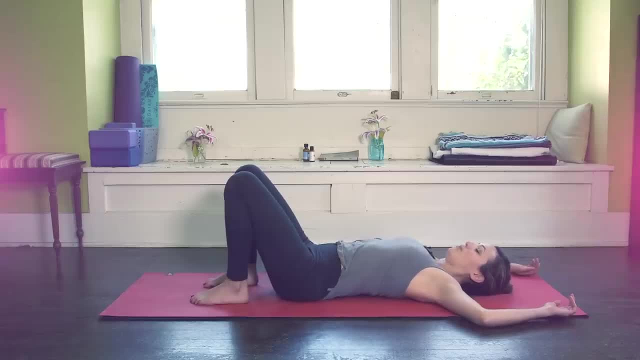 up finding a little soothing movement for that lower back, staying grounded to the soles of the feet. Just do a couple more, stretching the belly long as the lower back lifts up and then maybe drawing the navel down as we lengthen through the tailbone. lower back flush with. 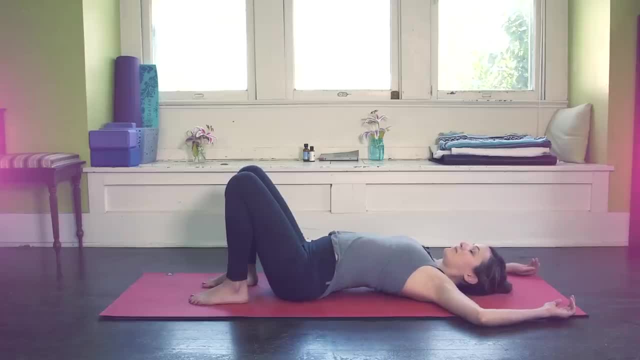 the mat. Do a couple more on your own. It's like a baby bridge, Baby. The bandhasana experience- Cool. When you feel satisfied with that, I got a little zend out there. When you feel satisfied, we're going to lift the knees back up and we're going to cross. 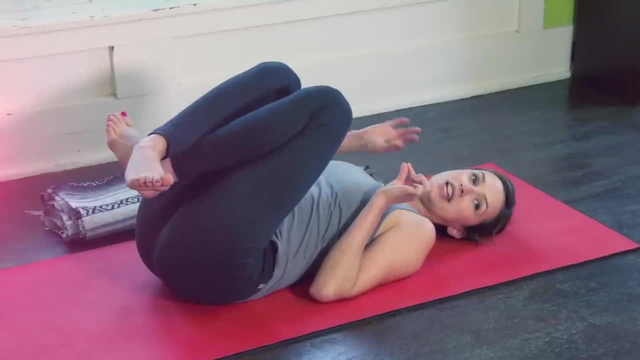 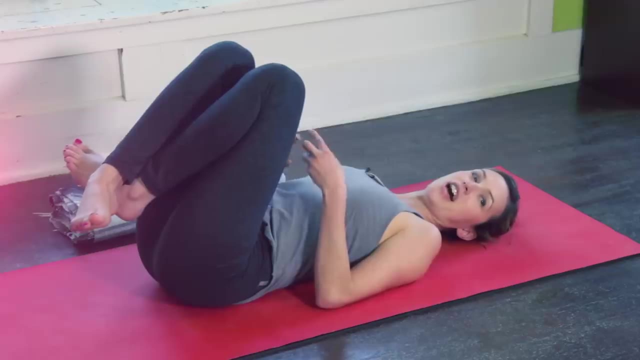 the ankles and we have an option here. If you're really tending to lower back relief, skip this Rock to one side and come sit up If your lower back feels tight and you feel like this might be good. join me in a little. 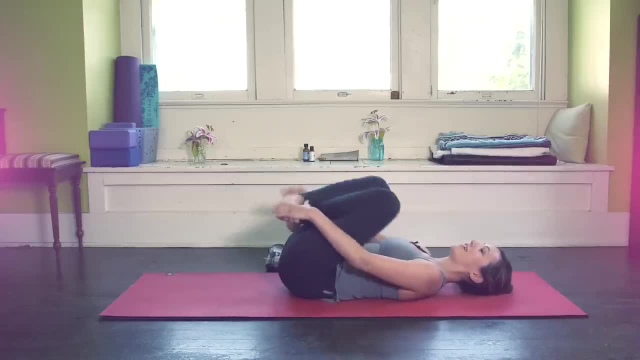 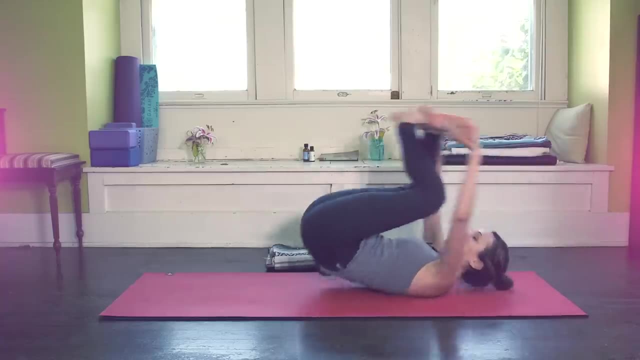 rock and roll up. So I'm going to grab the outer edges of the feet. I'm going to begin to rock a little front to back. If it feels like that's yummy, do it a couple times, massaging the spine. Remember, it's all connected. 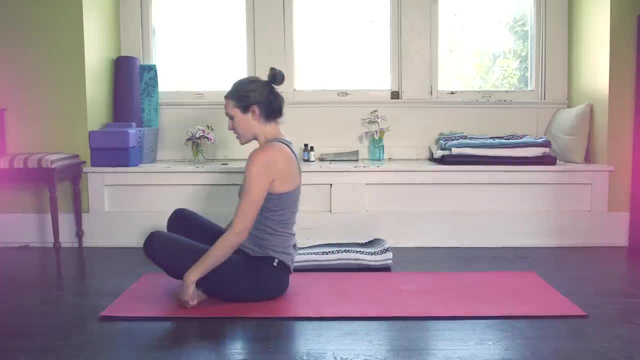 This is a great way to just kind of relieve tension and stretch and soothe the spine. Now, if you're a little more sensitive today- again, we're all different, approaching this different- then just skip that move and come to cross-legged position, which is where we 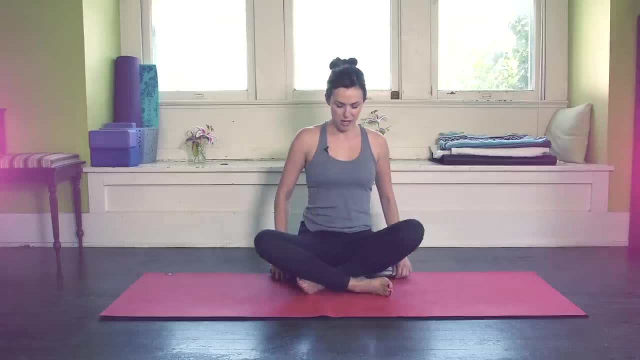 will all meet. I have a blanket here, conveniently. I'm going to lift my hips up on. You can use a towel or blanket. We're nothing at all as we come to cross-legged and bring the palms to the knees here. Nice and easy breezy. 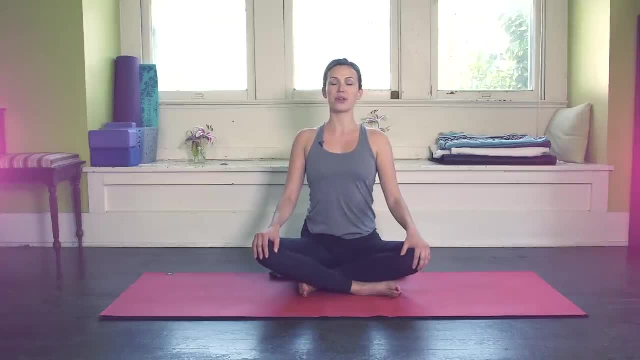 We inhale, press the palms into the knees, extend through the crown of the head, lift your heart chest open, Then on an exhale chin to chest navel draws back towards the spine. We come into what I call Mr Burns pose here rounding forward. 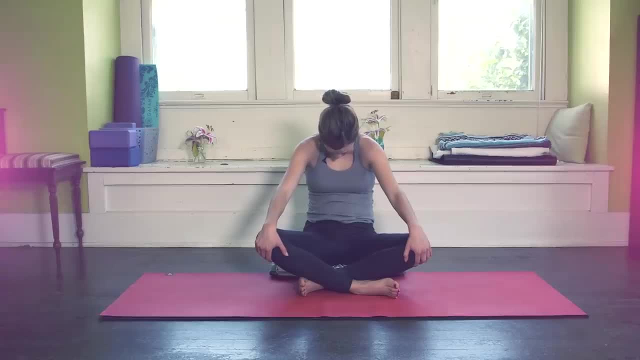 Breathe, Breathe into the back, Good, Good, Good, And then inhale, extend, tagging a little weight in the elbows here, Open the chest, the heart, And exhale same thing, chin to chest, rounding forward. 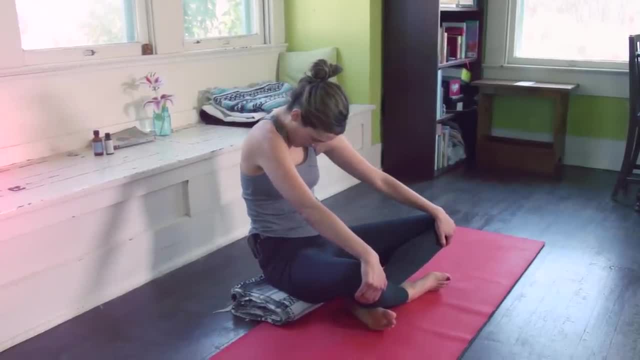 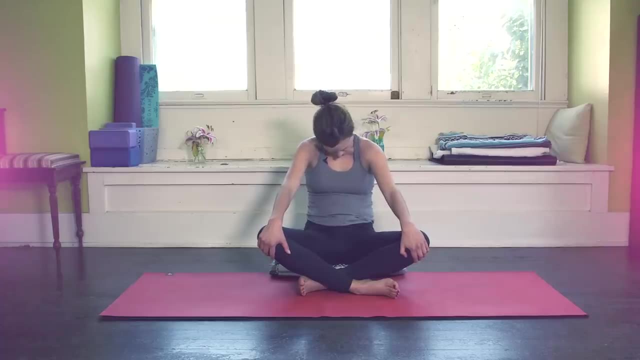 Go ahead and catch the weight in the palms And take a couple breaths here, Stretching the skin of the back. The breath can be so healing. so take some nice long, smooth, deep breaths here, Good, Good. 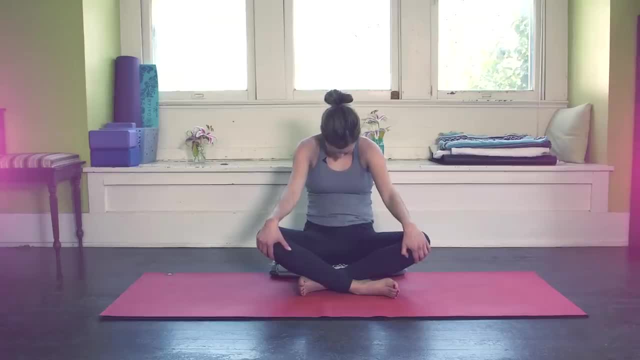 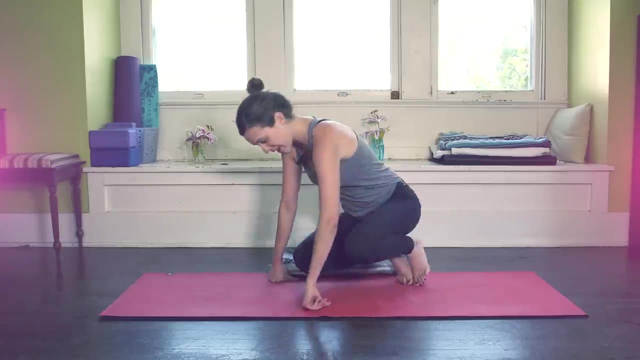 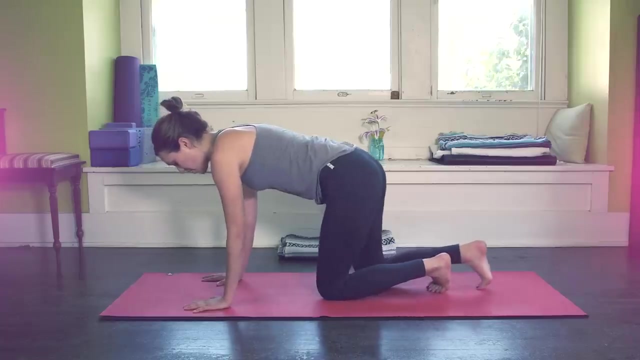 Good, Good, Good Good. And then, slowly, we'll rock all the way back up and come to all fours. Nice and slow, Take it easy, Honor the body, Enjoy this practice this time. So we're going to come to all fours. 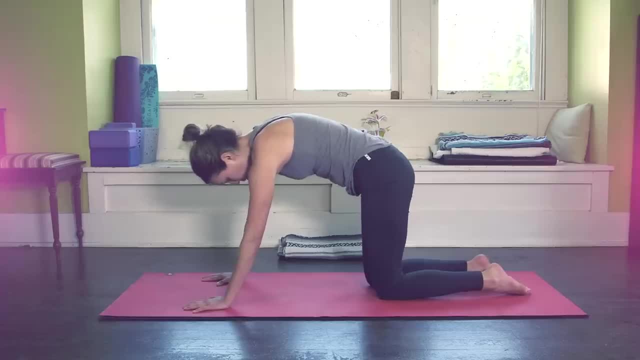 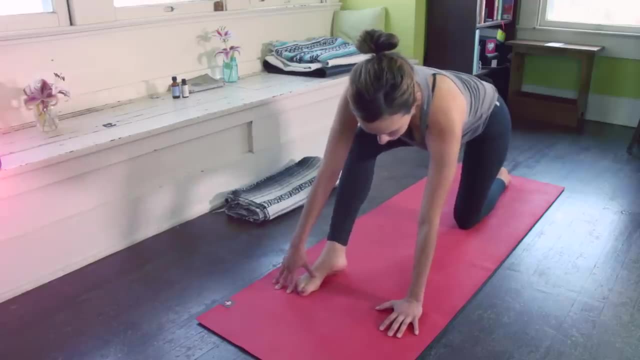 If you want, you can sneak in a gentle cat-cow here And we're going to take the right leg and lift it gently all the way up into a lunge. Good, Good, Good. Now again, if the lower back is tight, breathe deep. 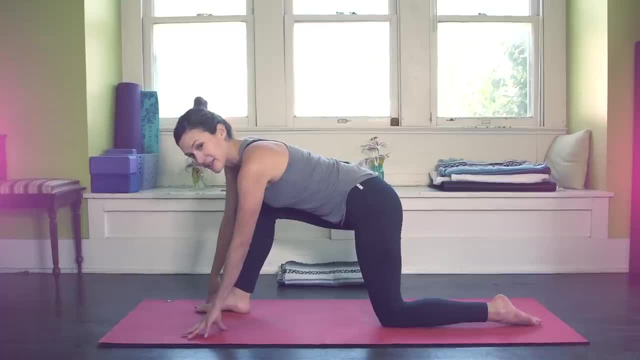 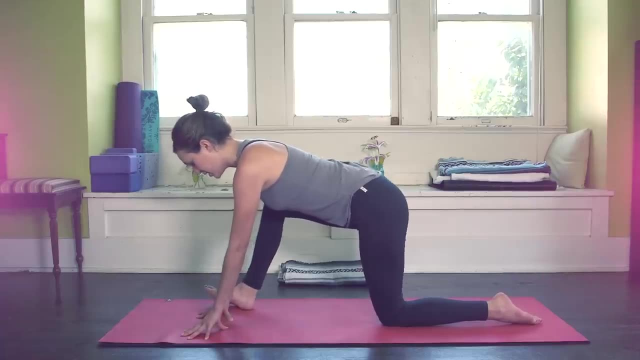 If the lower back is tweaking, you might save this. I mean, I just don't want anyone with lower back pain to do anything that they don't want to do, so just listen to your body and breathe. I'm going to heel-toe, heel-toe- my right foot out a little bit wider than I would normally. 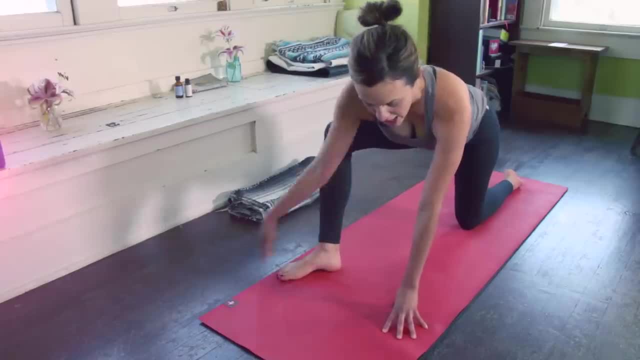 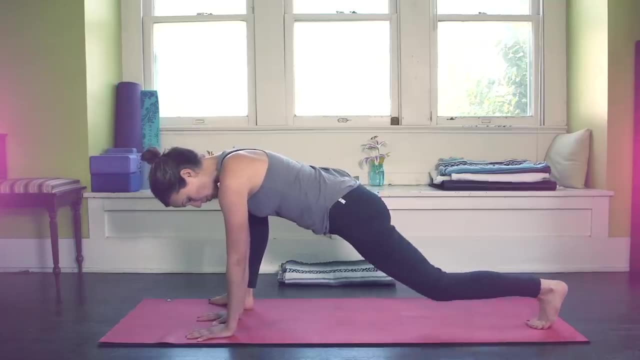 in a runner's lunge. You might even turn the right toes out slightly And we're going to bring both palms in towards the center line. Now I'm going to curl my left toes under, Walk my left knee back And slowly sink into the hip. 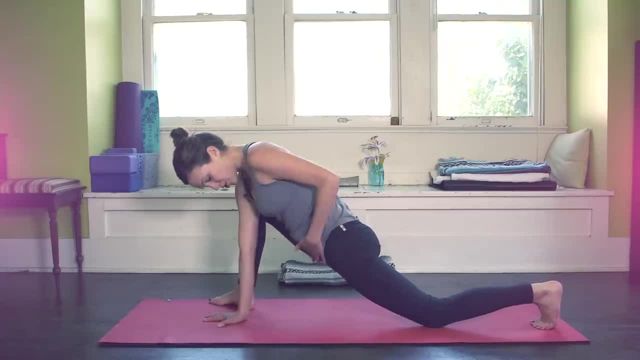 So what I'm doing is- this might seem a little counterintuitive, but I'm stretching the front of that left hip crease, the psoas here. that wraps literally from here to here, which often causes some crappy crap in the lower back. 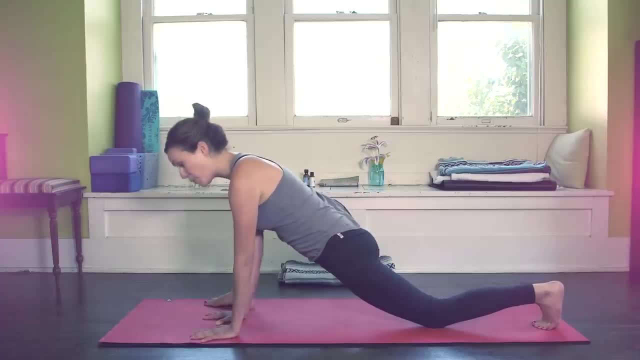 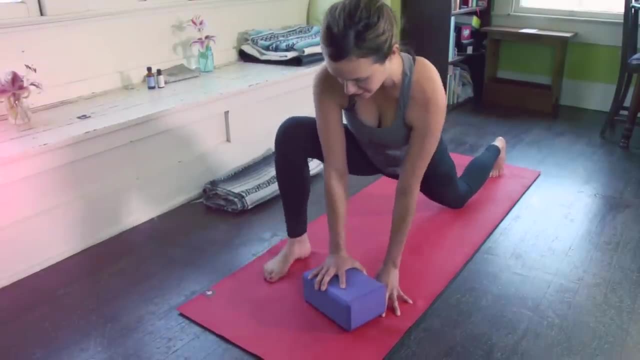 So we're finding a nice opening in the front of that hip crease. We have the palms here to support us. If you want, if you have a block or a book and this is just too much for you, you can lift the earth up to you, baby. 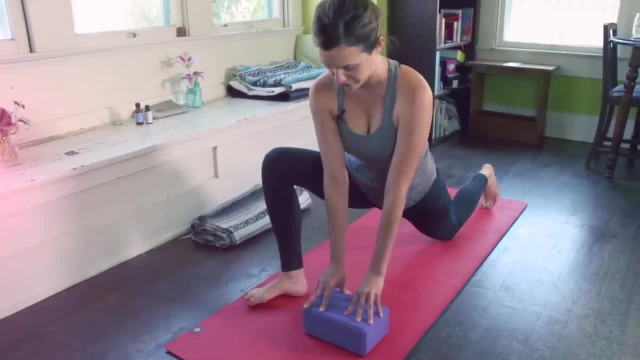 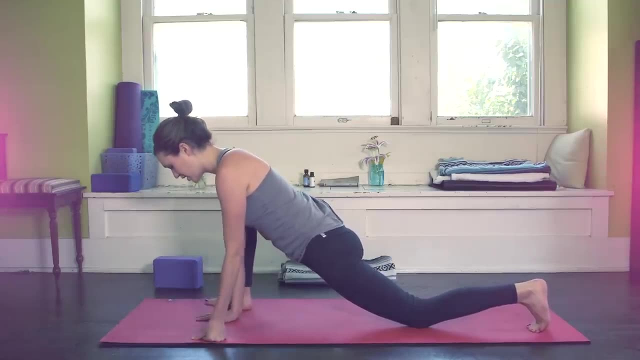 Yeah, Or fingertips is always good. Now breathe, Finding what feels good. Again, we're focusing on deep breaths and opening the front of that left hip. crease the psoas. If it feels right, you might lift that knee for a pulse or two. 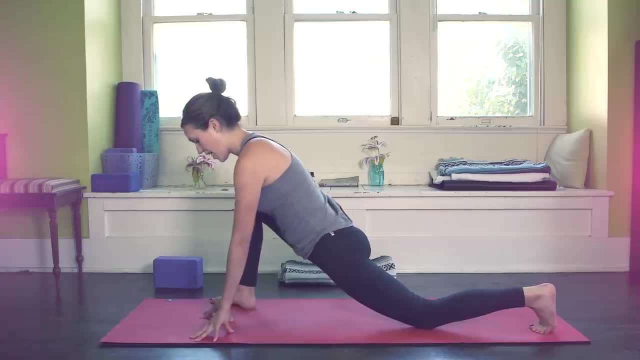 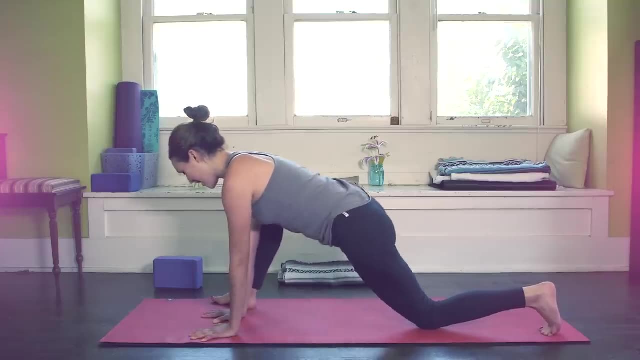 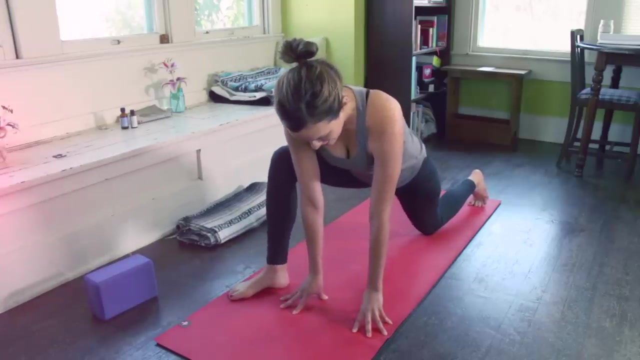 But if we're super tight then that might not be an option and you might stay up nice and lifted Couple more breaths here. Smile, We've got the skin of the face. We got this Then to come out. we'll come on to the fingertips. send the sit bones back for a little stability. 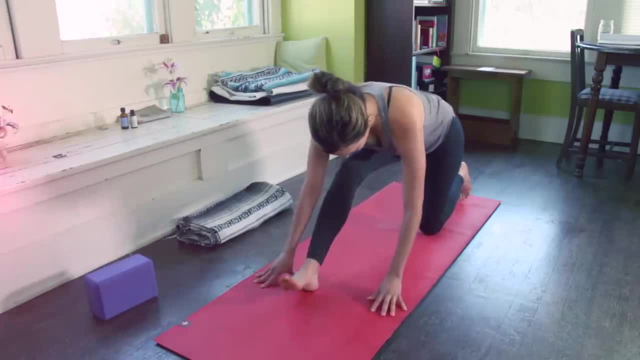 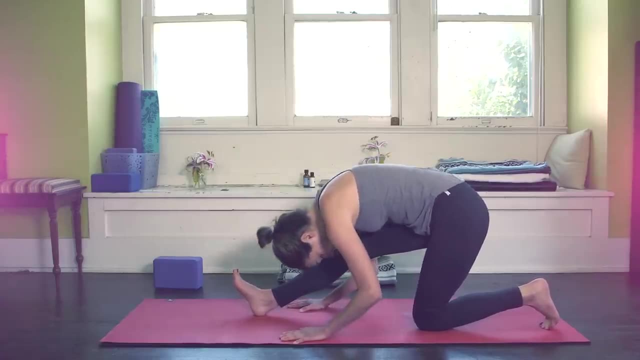 as we walk that right heel in, and then we're just going to take it for a nice little counter pose here. Right heel stays in the earth as we relax the weight of the head over, pulling the right hip crease back. This doesn't have to be a deep stretch, guys. 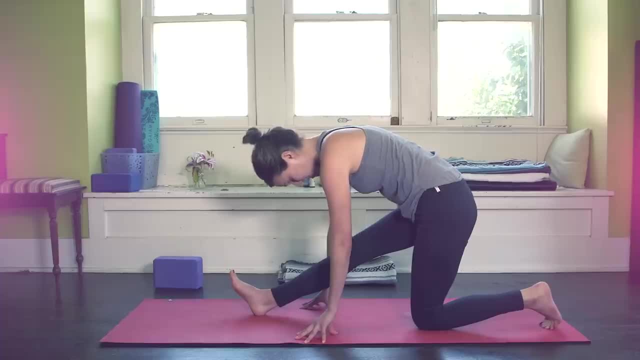 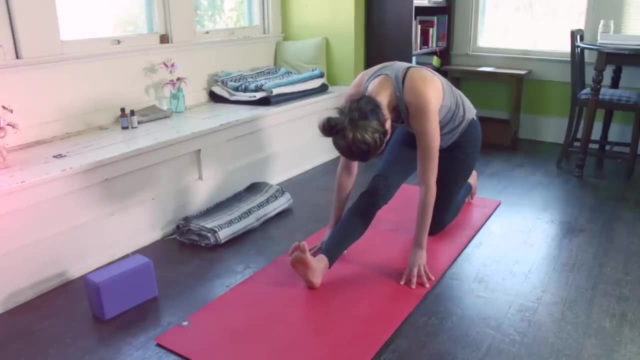 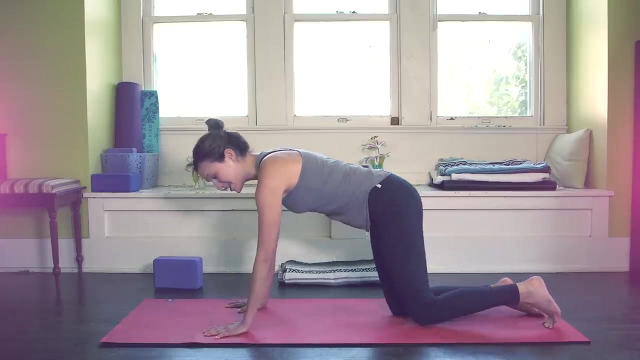 In fact, if we're tending to the lower back, we should keep it nice and spacious, nice and easy. So one breath here, with the weight of the head over, Remember it's all connected. Cool, Then we'll rock back onto that right foot, come to all fours and, nice and easy, gingerly. 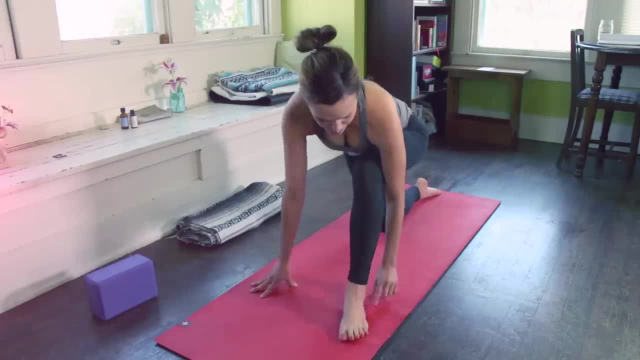 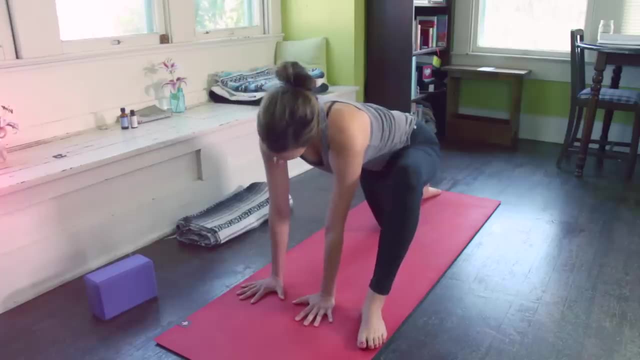 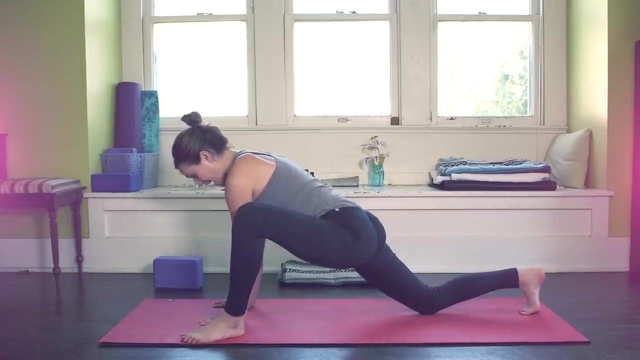 switch to the other side. Cool, So I'm going to heel-toe, heel-toe- the left foot out. now Both palms come in towards the center line. Take it nice and slow, find integrity, And then I will curl the right toes under, walk that right knee back and check out what's. 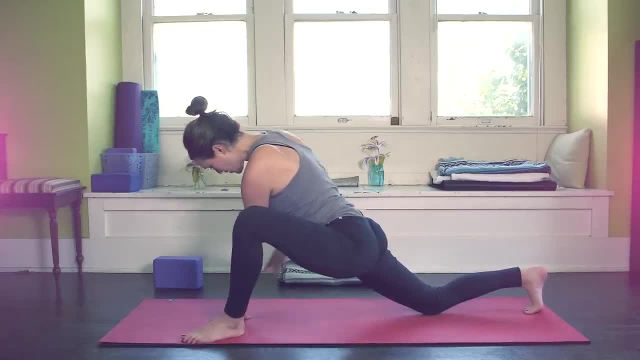 it like on the other side. So again I'm focusing on the psoas muscle, or we can just kind of bring your awareness to the front of that right hip crease, Stretching it nice and long. using the breath to breathe here might lift that back knee. 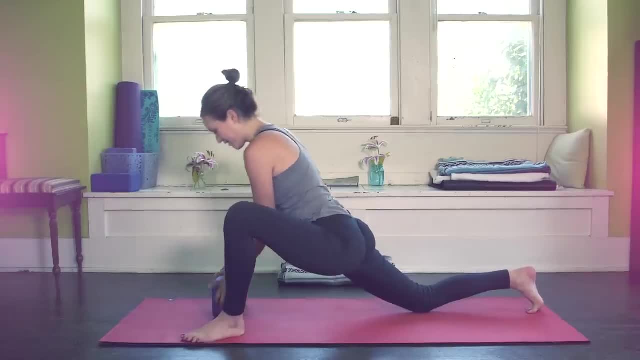 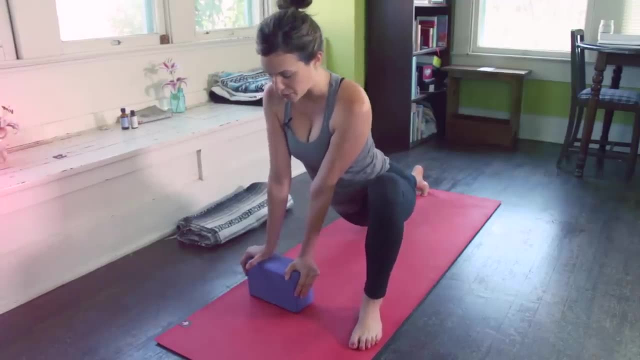 Again, as we said before, we might lift the earth to us if it's really tight. That might be why your lower back is hurting. So opening up through the front body a little bit to provide relief and space for the lower back Ding. 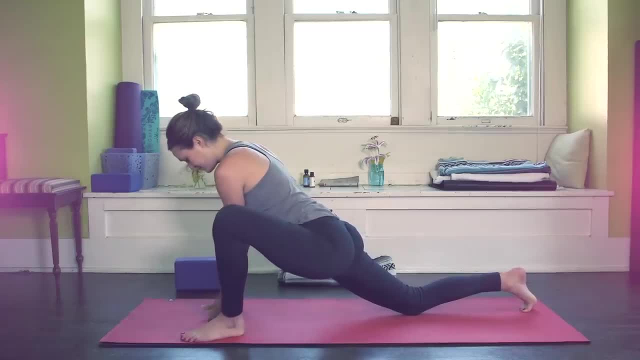 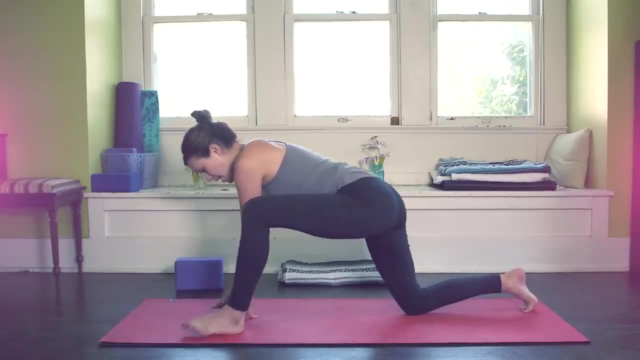 Okay, one more nice, long, smooth, deep breath here and then we come out, Nice and easy, lifting the sit bones back, walk the left heel in towards the center line and release over Again. we're not sinking all the way back. 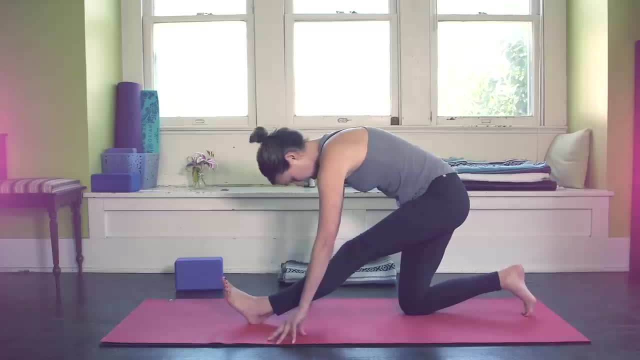 This isn't power yoga, We're just checking in, So keep a nice spacious vibe going on here. Weight of the head comes over, We breathe, And then the other side Good, Good, Good, And then we roll through the left foot. 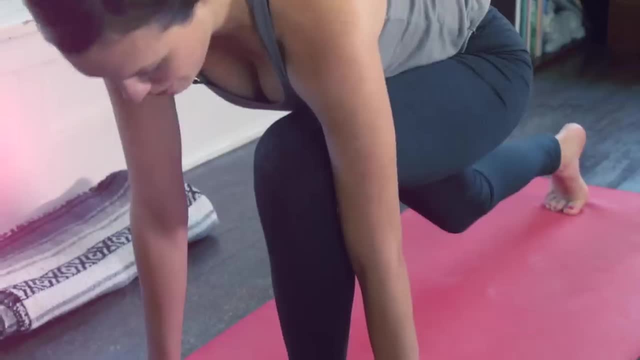 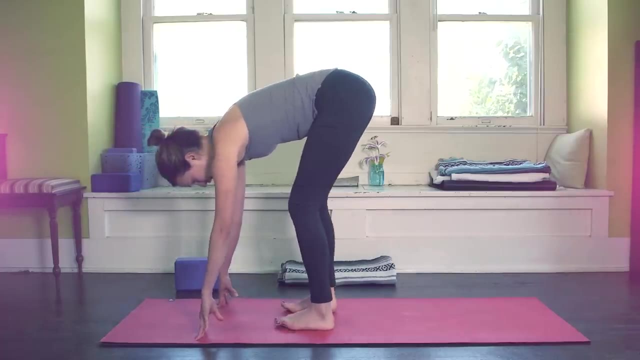 We use the fingertips for stability, and this time we're going to step that right foot all the way up to the left for a forward fold. Now, rule of the game here is: please, please, please, my friends, keep your knees bent. 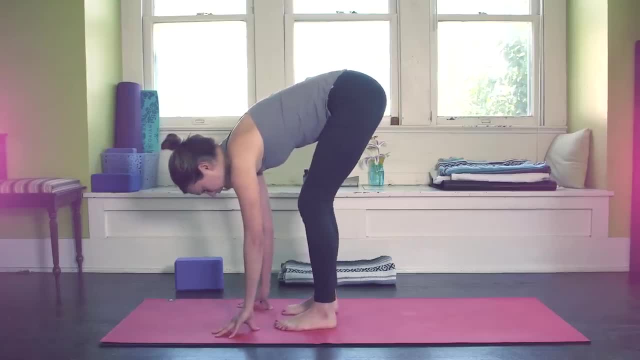 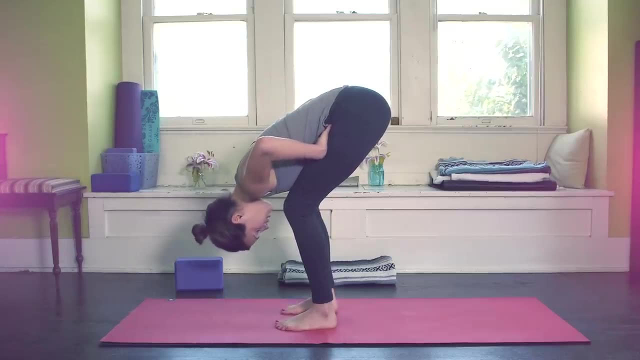 Bend those knees, Keep them soft. They can be super bent generously. Then I'm going to take my hands to the belly, draw the belly in just slightly and let the weight of the head hang over gently. Oh yeah, baby. 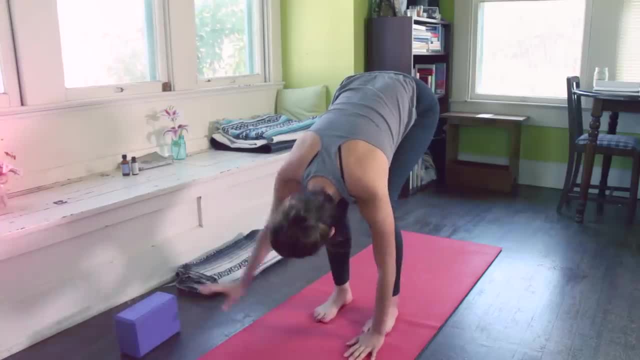 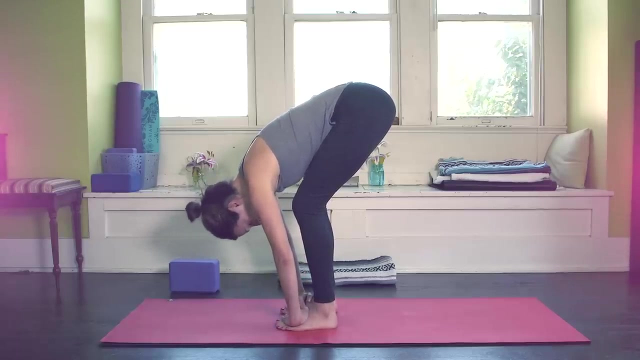 Release the fingertips. If you have a block, you can kind of rest it here, or a book. This is not about the palms touching the earth. They can go wherever they need. This is about feeling grounded through the soles of the feet and then finding spaciousness. 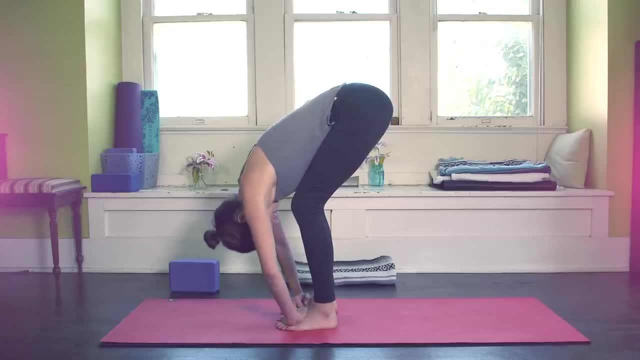 in the lower back. So we breathe here, We use the exhale to let go, We find a little weight in the sit bone, We release the fingertips, We release the palms And we use that inhale to maybe really feel expansion in the lower back. 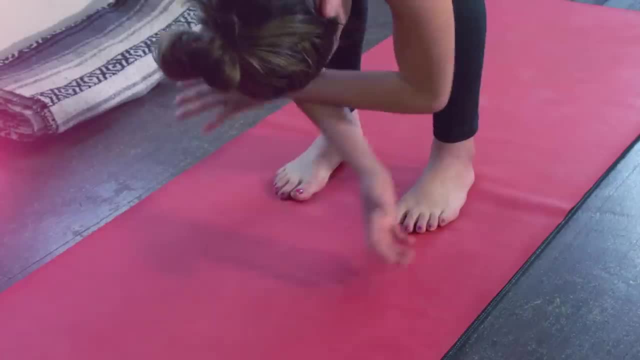 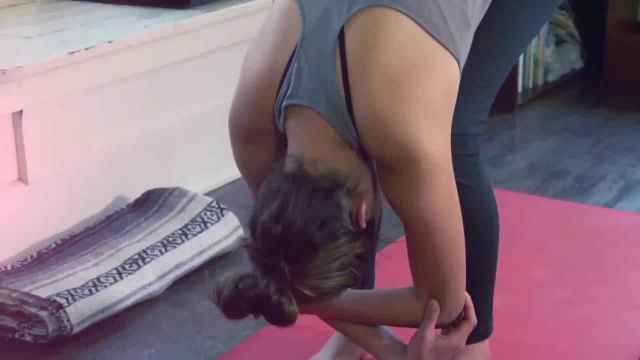 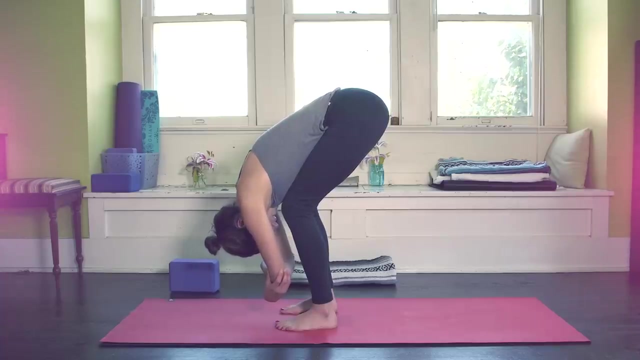 The exhale to ground down, find stability, Can grab the elbows here if you like. Let's take one more nice, long, deep breath in And then we let it all go To come out of this forward fold. today we release the palms or the fingertips to the 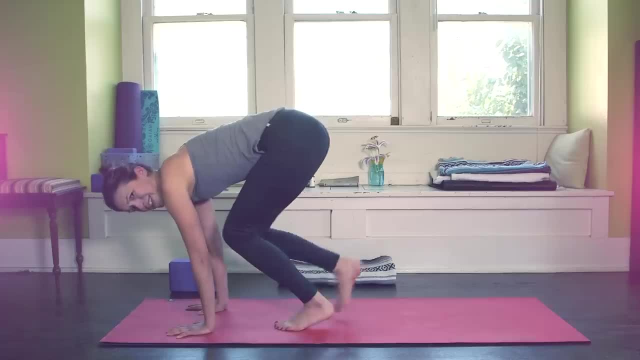 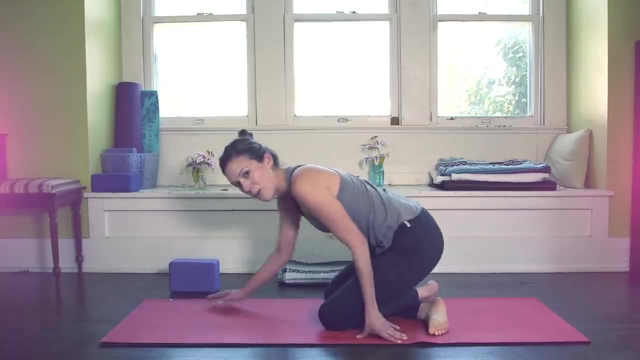 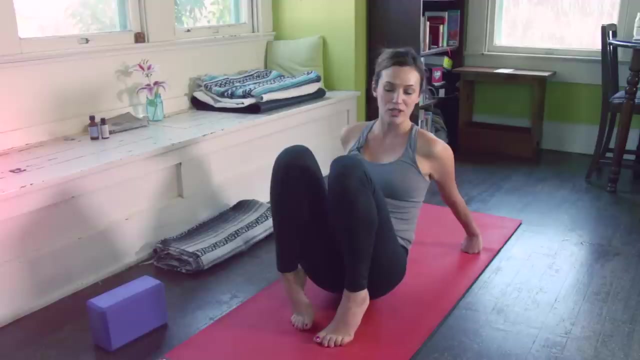 mat by bending the knees generously And then slowly- nothing fancy here. come back to all fours. Cool Cross the ankles. Nice and easy. We walk it back through Texas And come back to the back for our final posture, for the lower back. 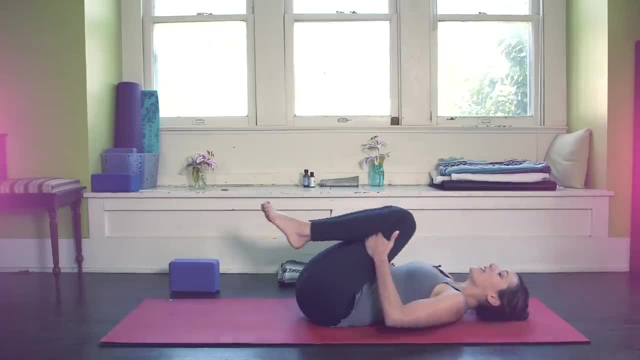 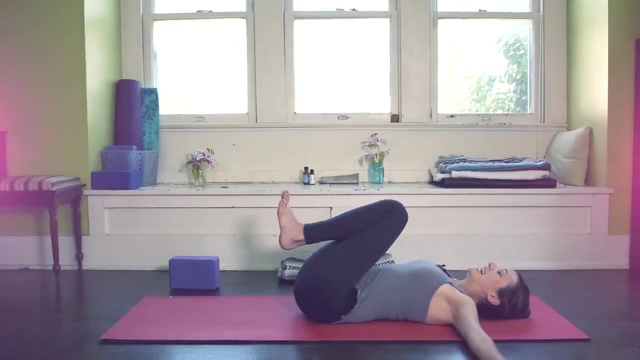 Yay, Hug the knees into the chest, Feel that space. Yeah, It's starting to feel better, It's starting to feel good And let go. And then we'll send the fingertips left to right- You know, I like to call this Texas T- And we'll scoop the tailbone up, draw the knees. 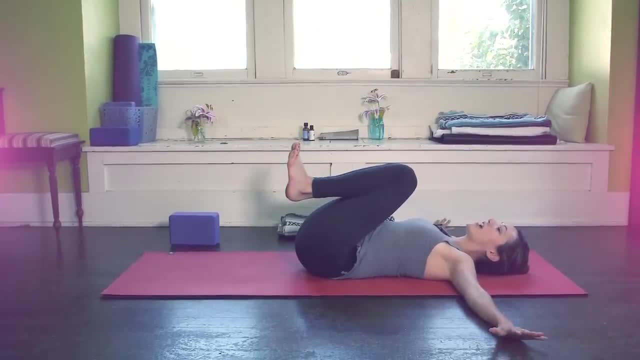 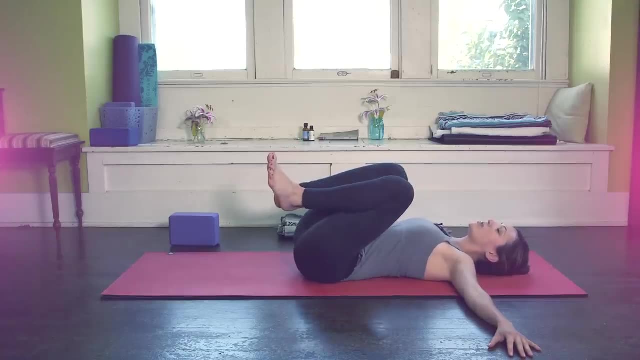 up towards the heart. And then this is not about forcing. This is about, again, gentle, finding ease, creating space in the lower back. So I'll gently melt the knees towards the right side And, rather than keeping the knees actively hugging up towards the heart like we normally, 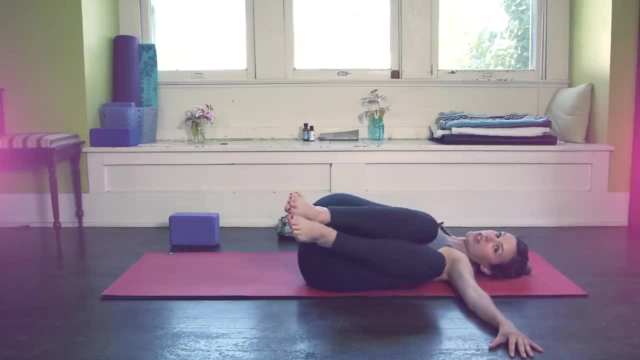 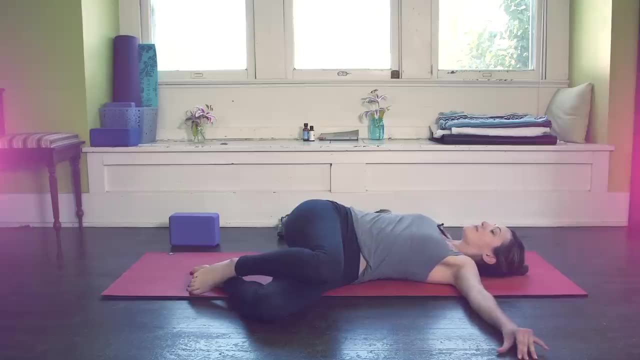 do give yourself a little more space. So again, rather than drawing the knees all the way up here There's ease. I'm letting myself have a little more spaciousness, a little more just ease. So I breathe here. I can take that left palm, of course, guide it a little deeper into the posture. 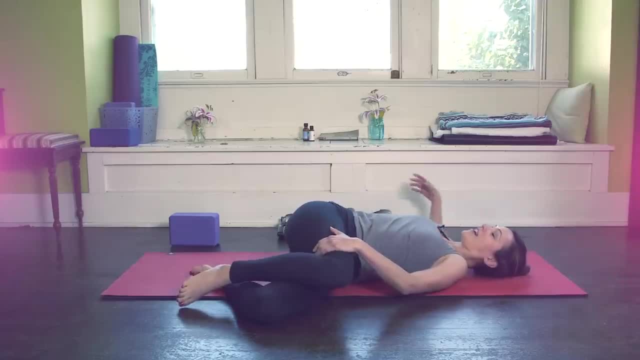 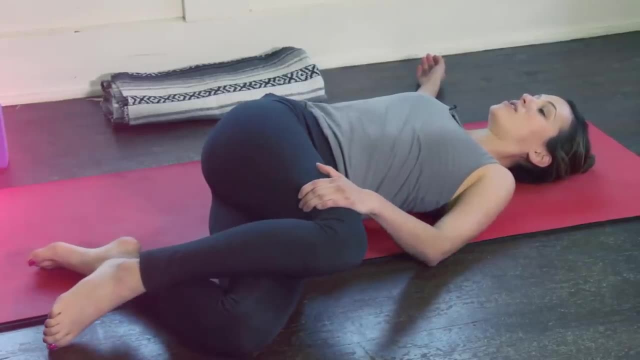 I'm breathing now again into that psoas lower back outer edge of the hip, Yummy. So I'm encouraging us to start here as a way of just again moving with ease. But you can of course, hug the knees up and play with that. 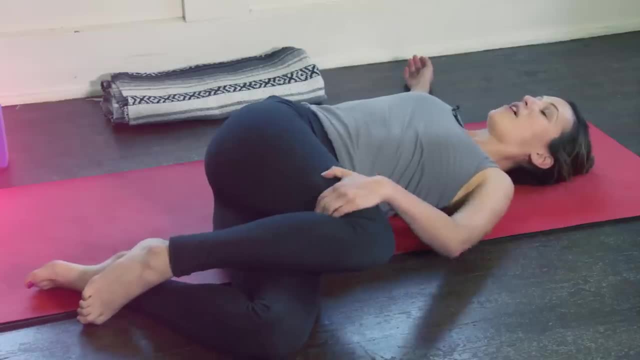 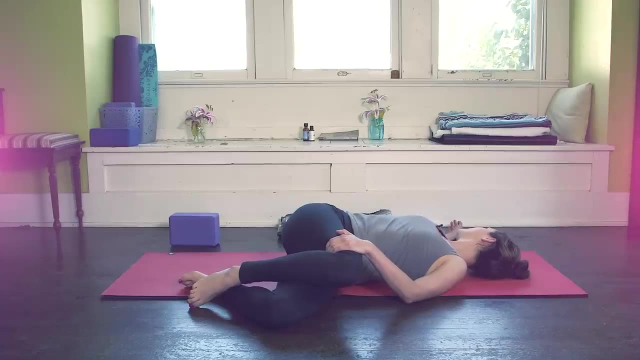 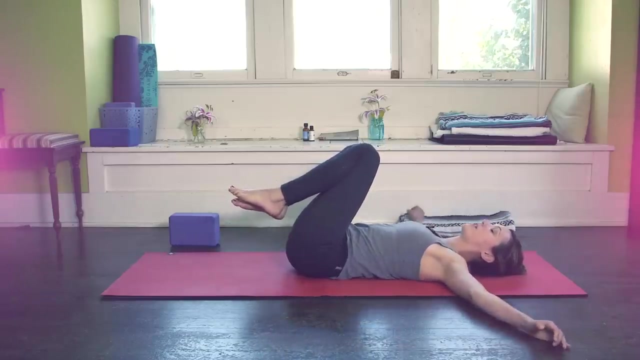 Yeah, You can play with anything in between. A couple more breaths here, You might turn to rock onto the right ear And then, on an exhale, nice and easy breezy. melt it back through center, Itch your nose, if you have an itch, and then send it to the other side. 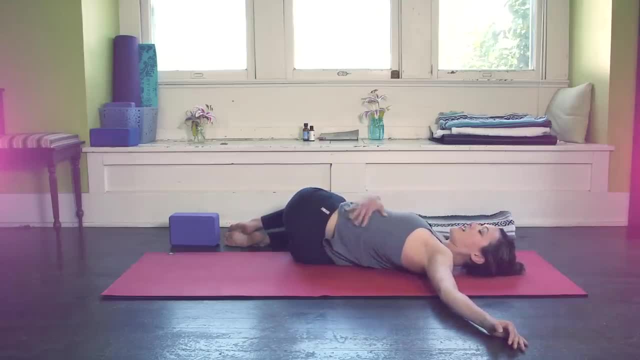 Here we go Again. I'm giving myself a little more space, Using the right palm to guide. I'm not anchoring anything, I'm just kind of letting gravity do its job. Nice, long, smooth, deep breaths. Turning onto the left ear. 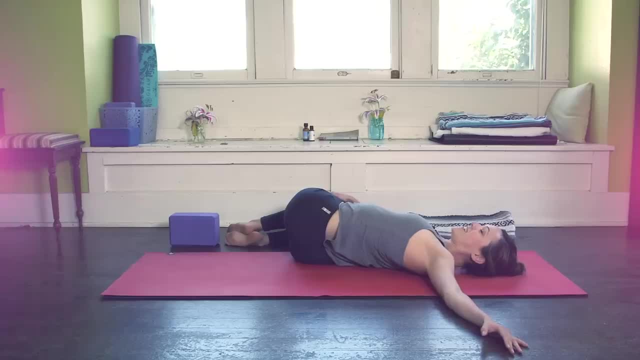 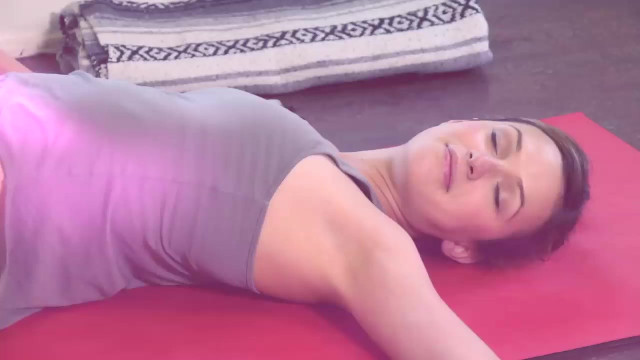 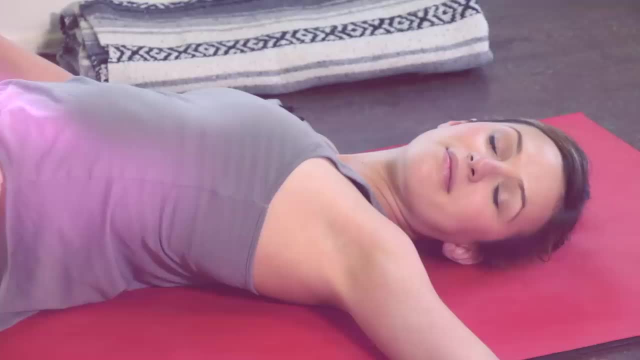 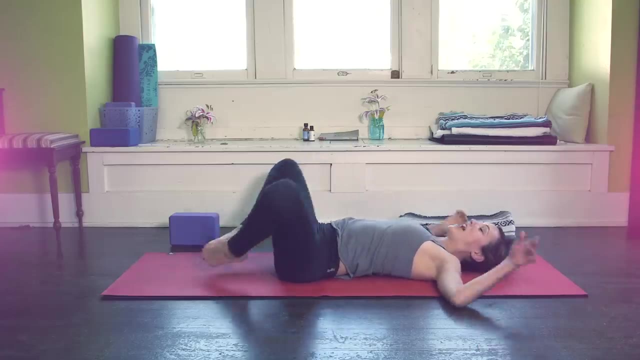 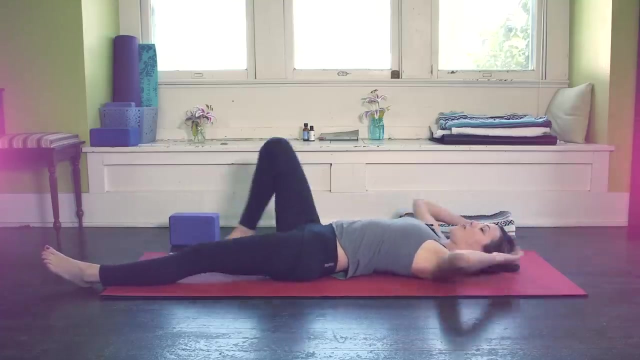 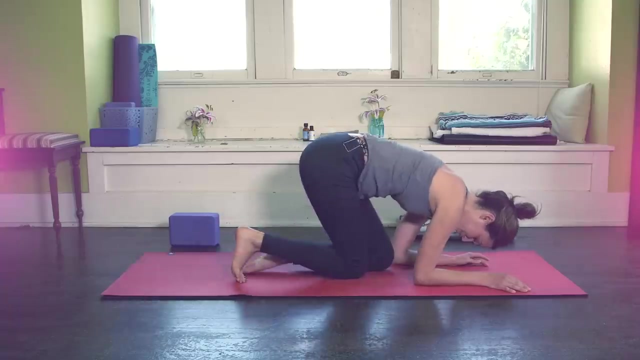 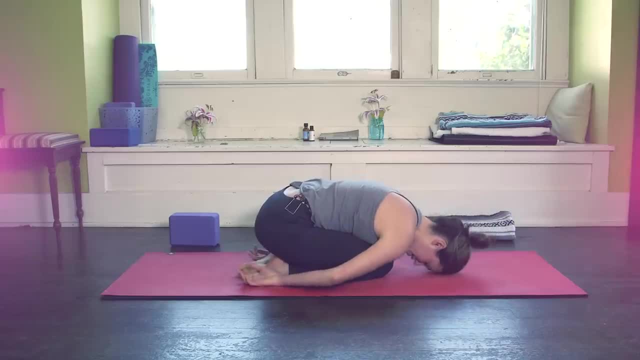 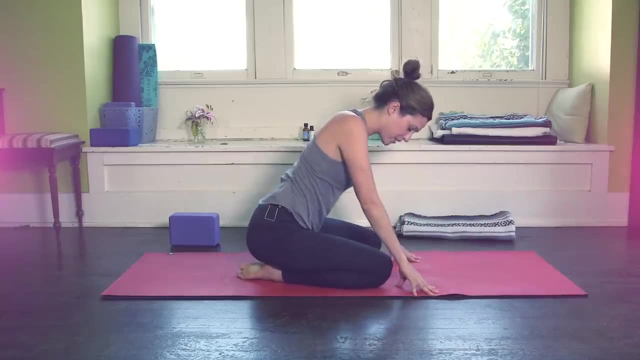 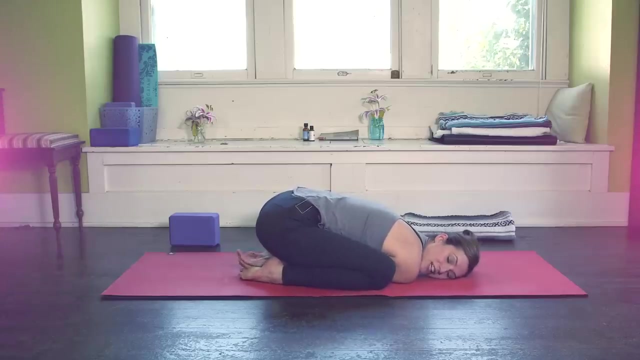